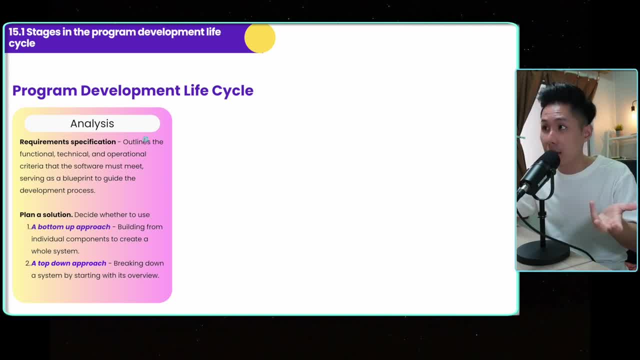 before you started coding on building the application, you will need to do some analysis on what the requirement specification is. So I have a definition here, but what it's saying is that you need to figure out what your. what is the problem that your application is trying to solve? 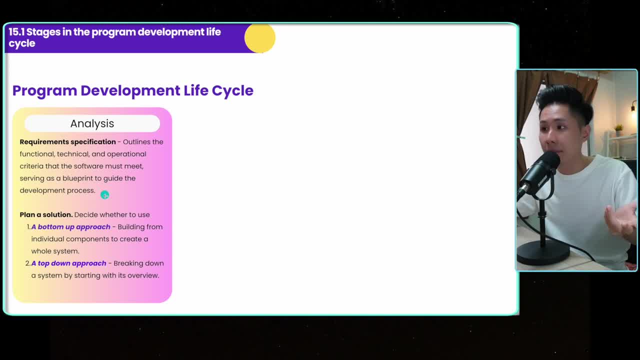 Or what is the convenience that it will provide and when you're planning a solution to reach your requirements. specification: there are two different approaches: A bottom-up approach, meaning you build from individual components to create a whole system, like a LEGO, whereas a top-down approach is by starting at this overview And after the analysis phase. 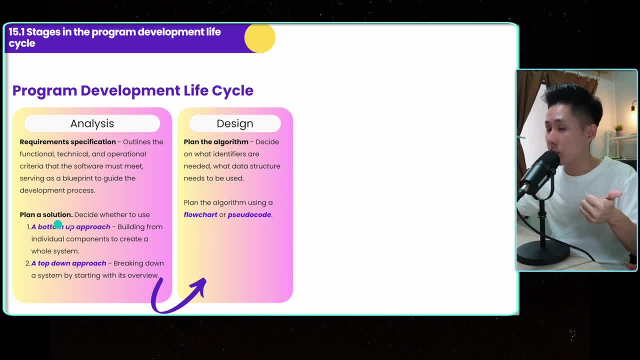 after you have decided what's the requirement specification and what approach you're going to use, you're going to plan out the algorithm to solve the problem. as learned in the previous chapter, we can plan the algorithm using a flowchart or pseudocode and that's everything that you do. 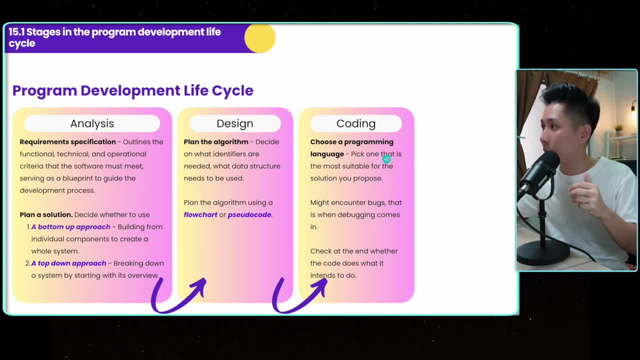 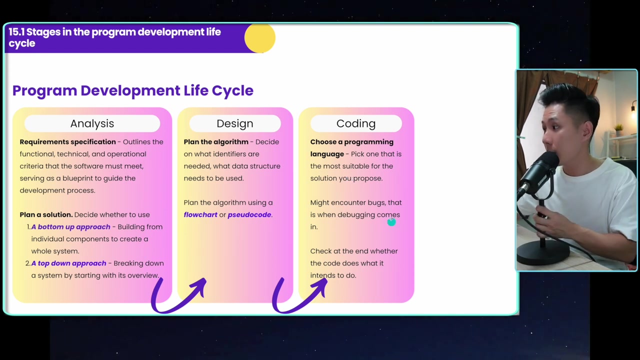 before you even start coding. and next one, which is when we started coding: choose the programming language. pick one that is the most suitable for the solution you propose. so, like the language we learned in language lesson, programming languages- different types of them. they do different things. so this is when you pick the most suitable one for your application. so you might encounter bugs, but 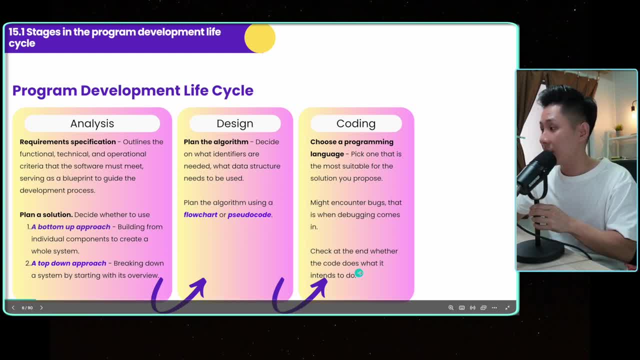 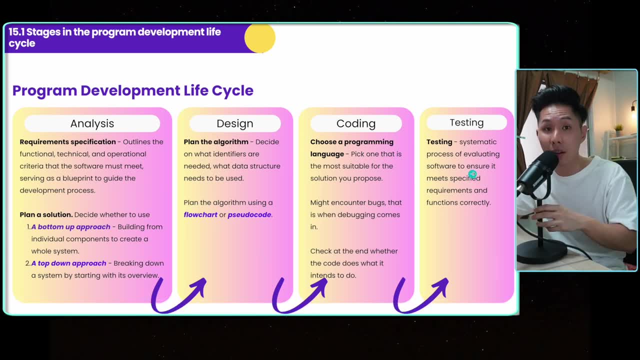 that is when debugging comes in check at the end, when the code does what it intends to do. so after you launch your software. before you launch your software, that should be when you test out whether it reaches your program requirement or not, and we will explore a few testing methods. 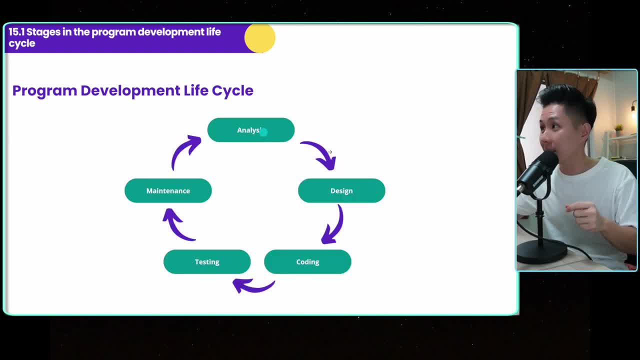 during the video as well. so this is the defenses cycle. there's a the reason why it's called a cycle. if you look here, it's because every time you implement a new feature, you have to go through the analysis phase again. this is also why every application that you download on your phone- 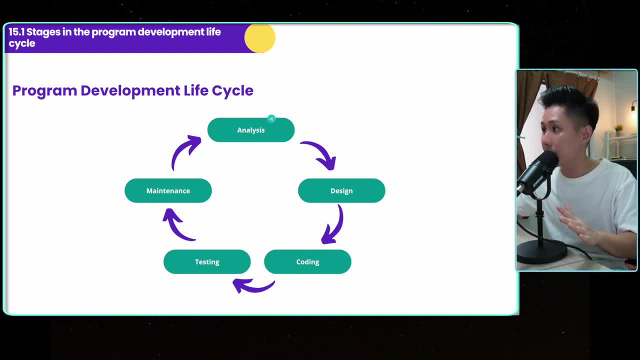 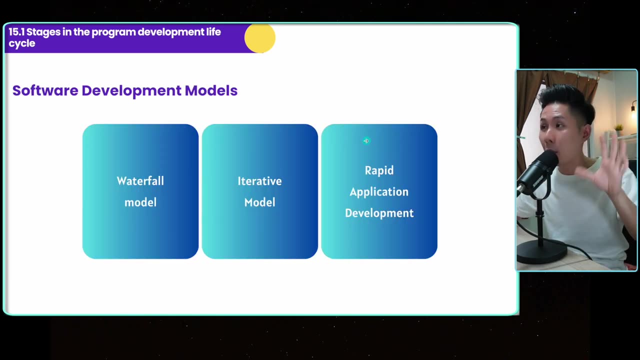 they require software update because the software developers, after an analysis stage they figure out at- oh, maybe i'm starting again- should add this feature. so this is why they do this all over again to implement the new feature in the application. so that's the cycle part of it, and i want you to to teach you about a few. 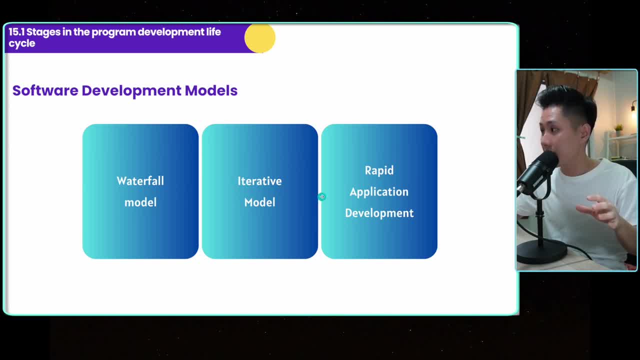 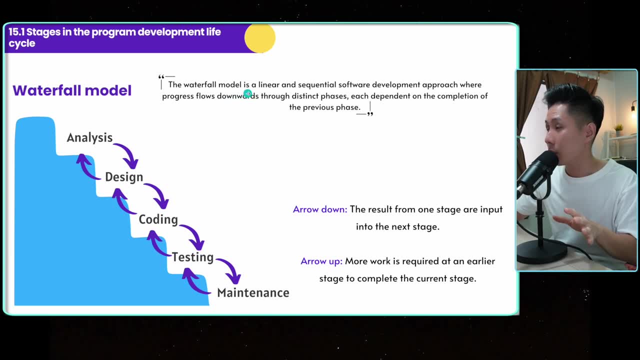 software development models: waterfall, iterative and replic application development. so let's look into one of them, one by one. the waterfall model is a linear and sequential software development approach. linear and sequential where progress flows downwards through distinct phases, each dependent on the completion of previous phase. so this is how waterfall model look like. 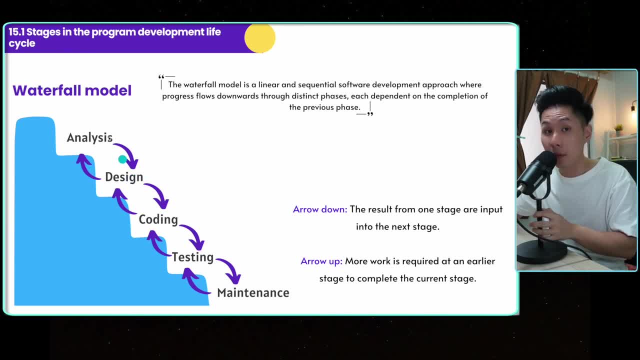 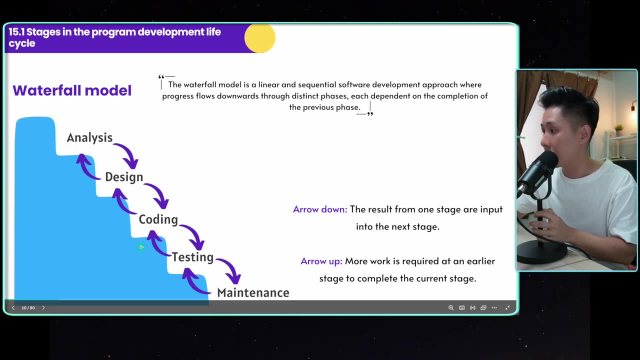 you can't do design before analysis and you can't do coding before design, because each stage relies on the previous stage. so error down means the result from one stage i input to the next stage and more work is required at an earlier stage to complete the current stage. 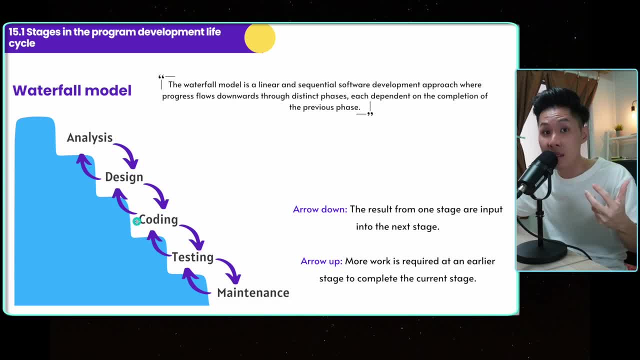 meaning you go back up because there's something that has not been done yet. now for waterfall model, i would describe it as a very rigid model, because once you start it, you just can't go back. you can't go from testing all the way back to analysis, because 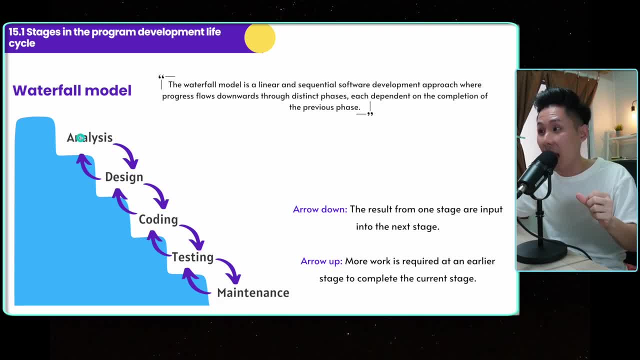 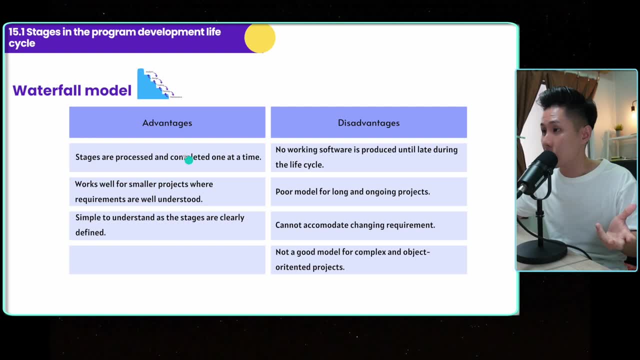 it assumes that all the requirements have been figured out and then you just follow this progress to create a software. but then it does have some advantage. advantages: stages are processed and completed one at a time, so there's no confusion on what stage we are in. works well for smaller projects. 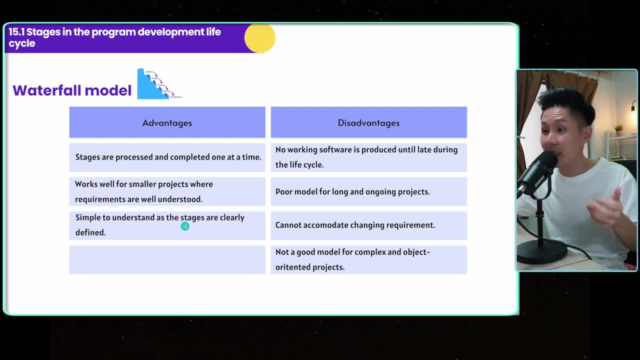 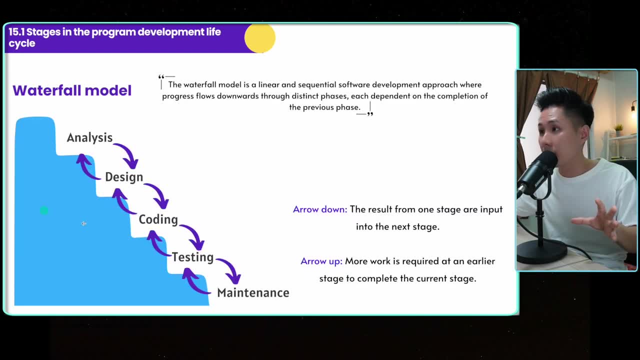 where requirements are well understood and it's simple to understand, as the stages are clearly defined, whereas the disadvantage is that you are not creating anything throughout this entire process. here, because the product will only be um shift ship after the testing phase and it's a poor model for long and ongoing projects because requirement requirements are not going to be. 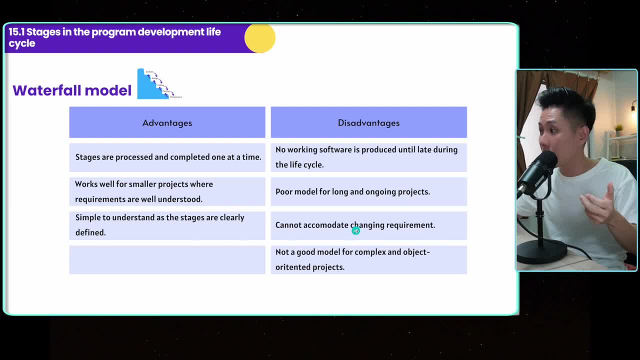 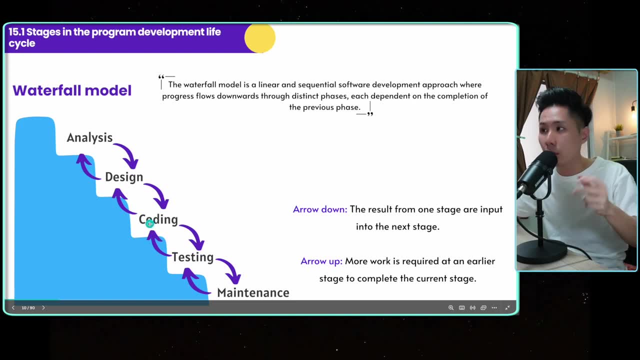 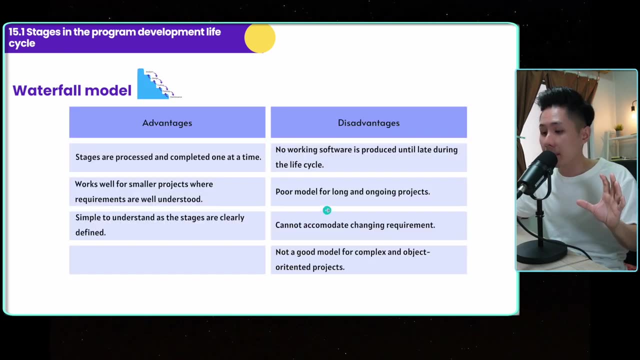 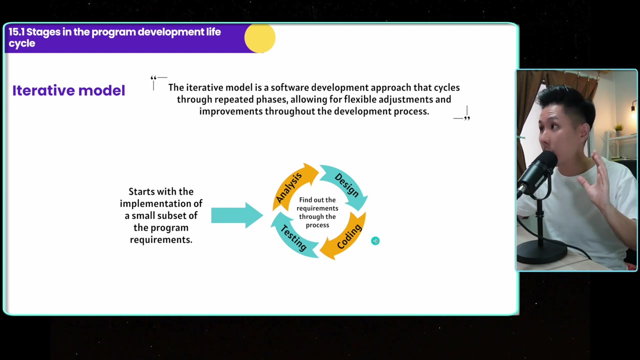 implemented in the future. so the third disadvantage is that the requirement might change, which is a third disadvantage- cannot accommodate changing requirement, which means that if, when you're in this coding phase already, you can't add more features because otherwise you have to go to level back up. so this is not a good model for a big project. this is why it stays here and an 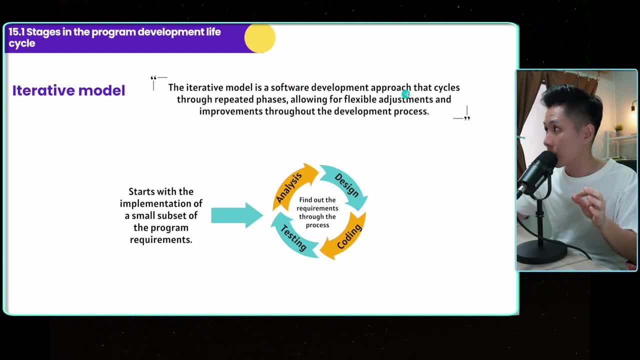 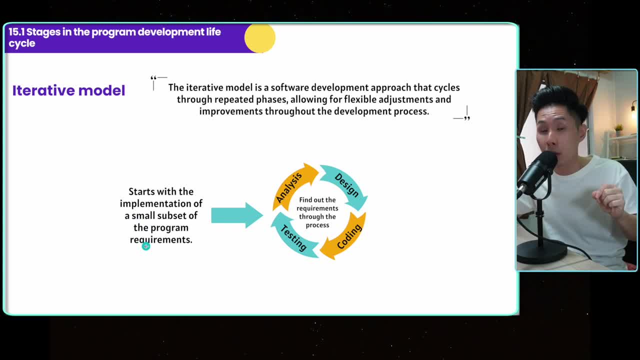 start with the implementation of a small subset of program requirement, meaning we create a smaller version of the software first, and then they only go through this analysis, design, coding, testing cycle many, many different times to add more features at a time. so instead of going all the way from the bottom to the top, they go to this cycle adding one feature. 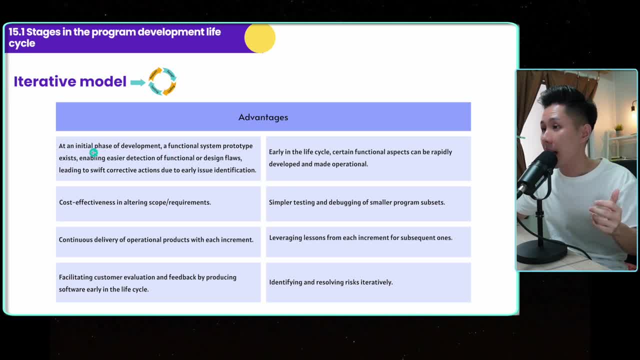 at a time. so the advantage is that at an initial phase of development, a functional system prototype exists, meaning you are creating a real product that the user or the tester can use, enable either detection of functional or design flaw, leading to swift correction corrective actions. so this is important and there's a principle in software engineering. 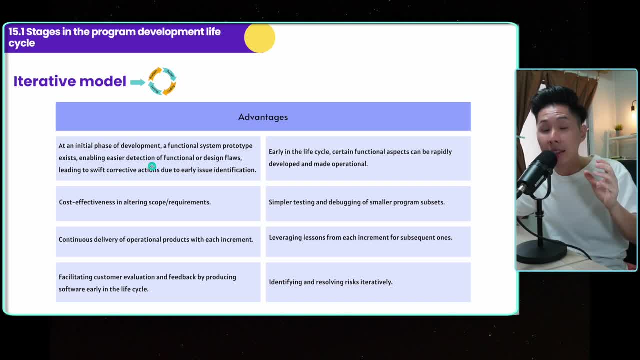 called fail fast, which means that you want to identify the errors in your code as fast as possible. iterative model allows you to do that because you are creating only a very small software, whereas the waterfall one where, when the error is detected, is usually a little bit too late. 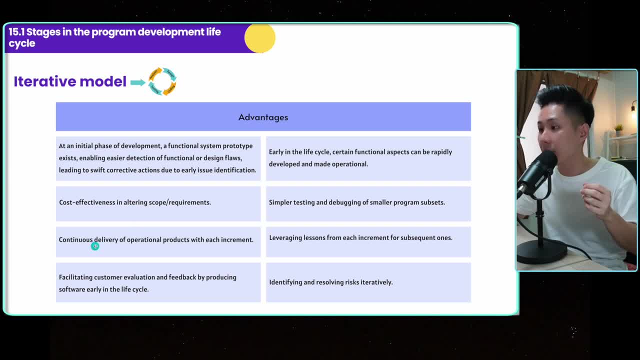 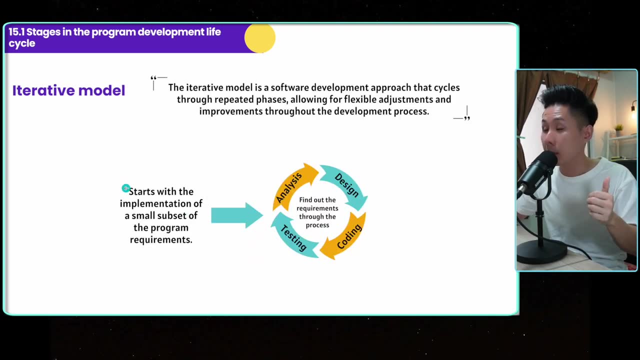 it's cost effective in altering scope and requirements continuously. continuous delivery of operational products with each increment, facilitating customer evaluation by feedback, by producing software early in the cycle. so what it means here is that the software development developer launched a small version of the software to the clients, to the 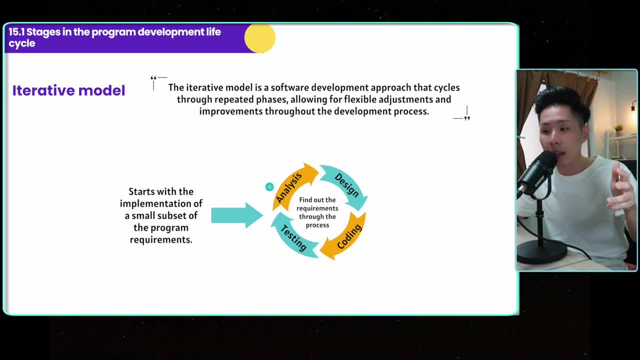 consumer and allow them to use it and test it. so this is important because customers will give you feedback and when they give you feedback, you can bring the feedback to the analysis, design, coding, testing phase to suit their feedback. so this is the one of the advanced technologies that we're going to talk about in this video. 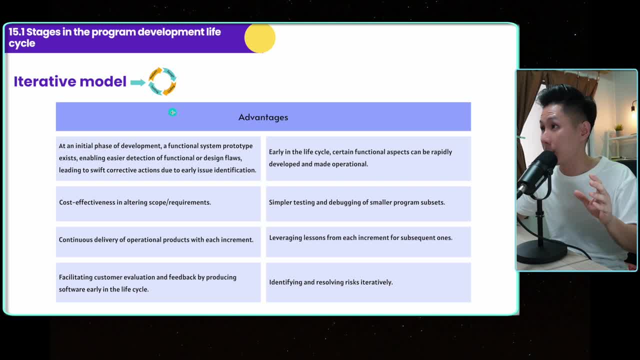 their feedback. so this is the one of the advanced technologies that we're going to talk about in this video. disadvantages of the iterative model, Whereas another one early in the life cycle. certain functional aspects can be rapidly developed and made operational: Simple testing and debugging. 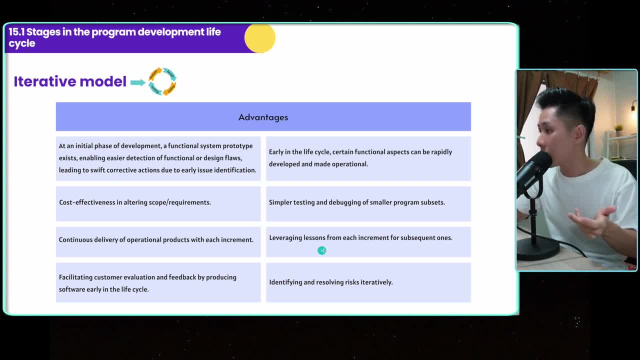 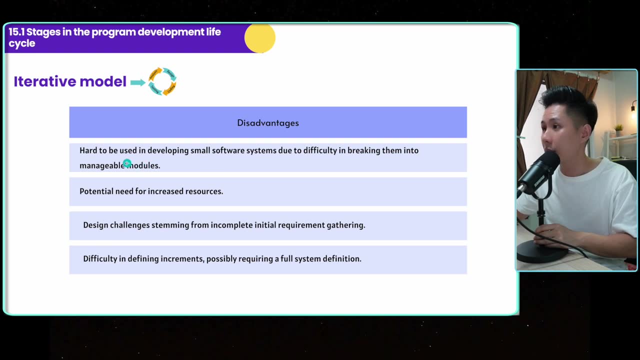 is, for the program is smaller, it's easier to test, Leveraging lesson from each increment for subsequent ones, identifying and resolving risk iteratively. So this is likely the model that you'll follow when you're creating an application in the future. Whereas the disadvantage is hard, 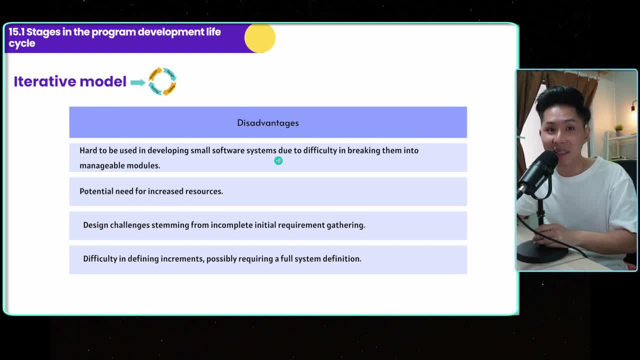 to be used in developing small software system, because if for a soft software system it's already small, So it would be better to use a waterfall model- And potential need for increased resources. design challenges stemming from incomplete initial requirement gathering difficulty in 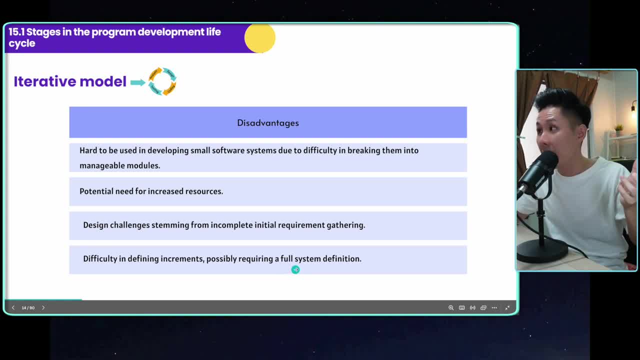 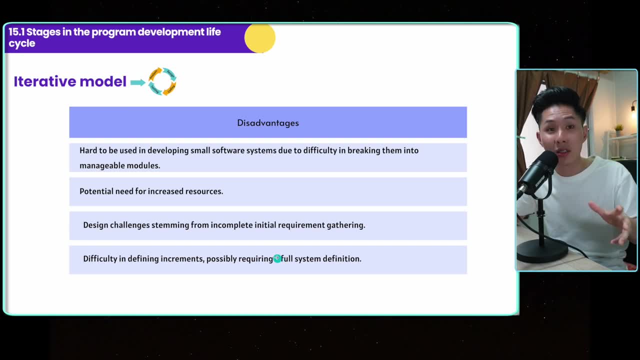 defining increments, possibly requiring a full system of definition, Disadvantage could be. what they're saying is that it could be very vague to the programmer on what you're actually wanting to create. So it's hard to be used in developing small software system because if for a soft 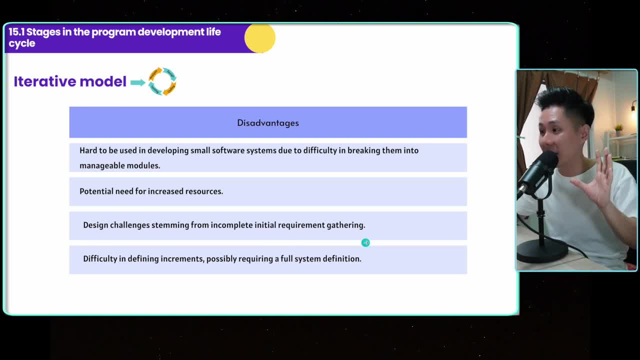 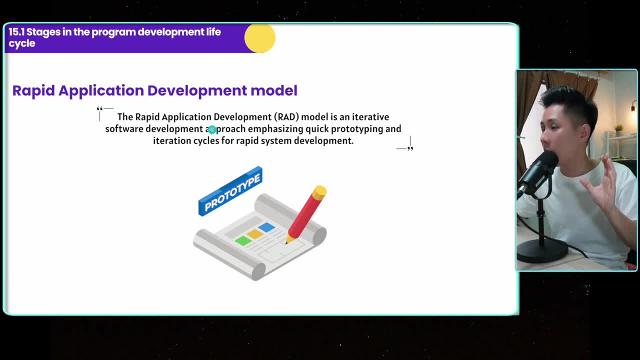 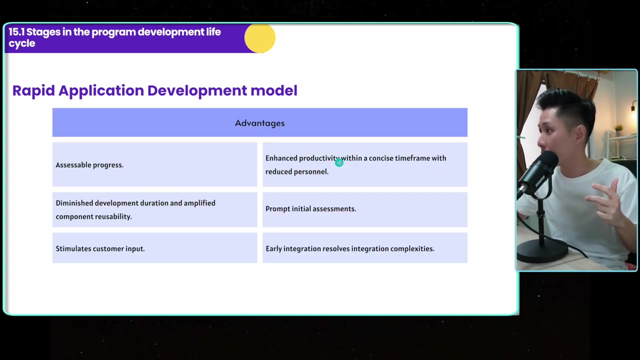 software system. it's already very vague to the programmer on what you're actually wanting to create. So because it requires consumers feedback, And that's iterative model. The next one is very similar to iterative model. It is called rapid application development model. It's an approach emphasizing quick prototyping, meaning you create a real product and iteration cycle for rapid system development. The advantages: assessable progress, enhance productivity. prompt initial assessment, diminish development duration. 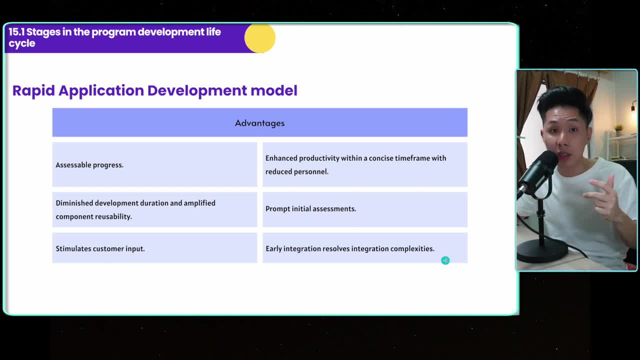 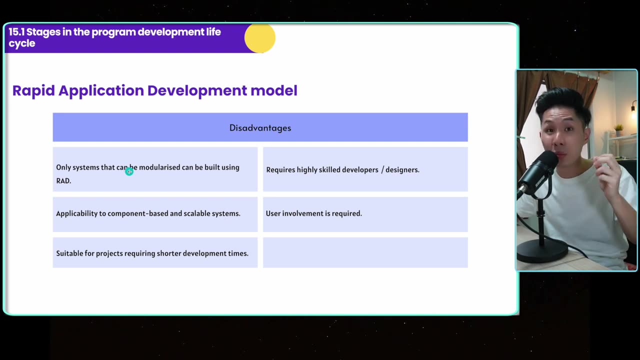 stimulate customer input. early integration, resolve integration complexity. So very similar to iterative model, but this one they create a real model as fast as they can, a prototype. So disadvantage only system that can be modularized, meaning that can be broken down into modules, can be built using RAD. applicability to component-based and scalable system suitable for project requiring shorter development times. User involvement is. 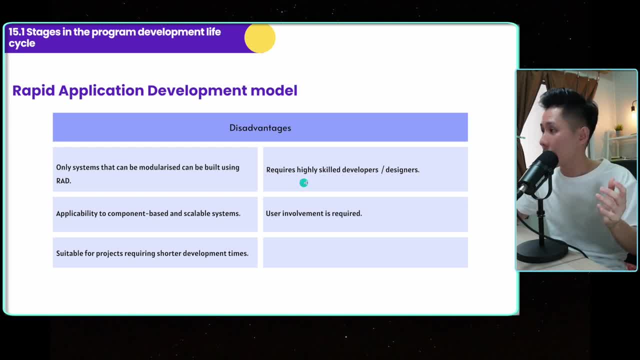 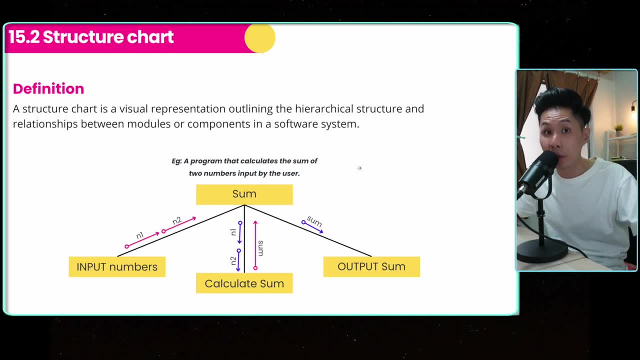 required. you need to find a group of people to test. your code requires highly skilled developers and designers. Now that's all about the different software development models. So now I want to teach you about the different tools that programmers use. First one is called a structured chart. It is a visual representation outlining the hierarchical structure and relationship between modules. Remember when we are coding in Python, modules are the functions that we create or the procedure in 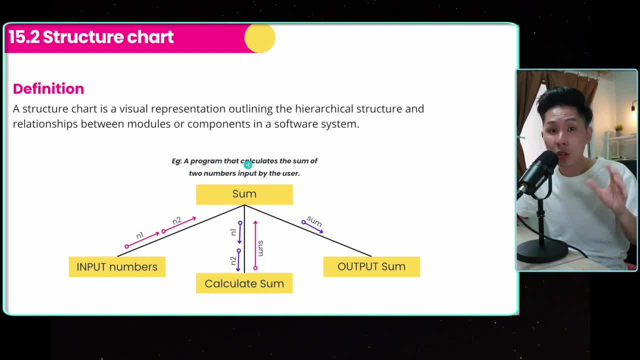 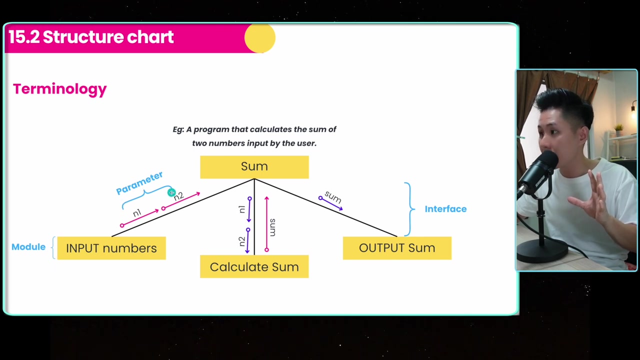 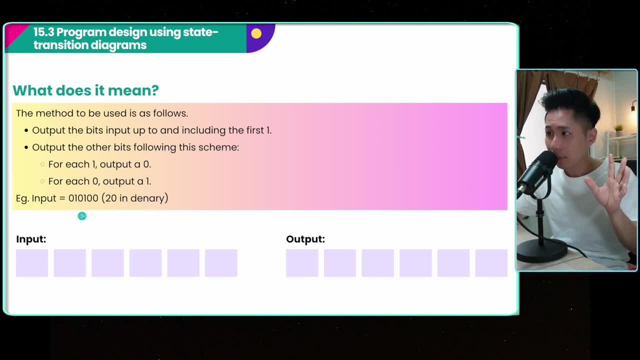 be very hard to understand. so let's do an example directly. the input I have is 0 1 0, 1 0 0. to convert it to dinner, is will be 20, so the goal is that I want to convert this 20 into negative 20 in. 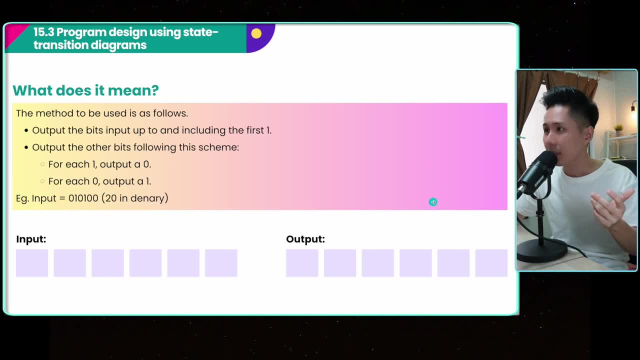 tools complement. using this game, using the algorithm, whatever the user input 0- I'm gonna output it. 0 until the first one, I'm still gonna output it, but that tells me that, oh, after the first one I'm gonna follow the other scheme. so for each one I'll put a 0, so input is 0 and output is. 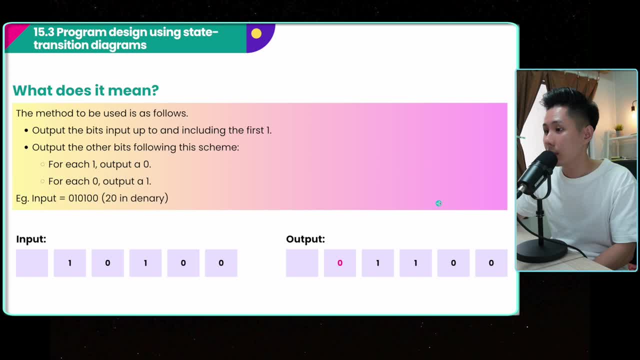 1 for each 0. so I'll put a 1, 1, y'all put 0, 0, y'all put 1. and if you were to calculate it using two complement method, you'll find out that, hey, using this algorithm, I already got negative 20 in two. 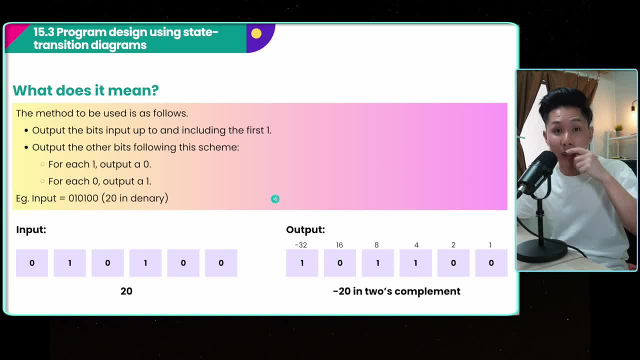 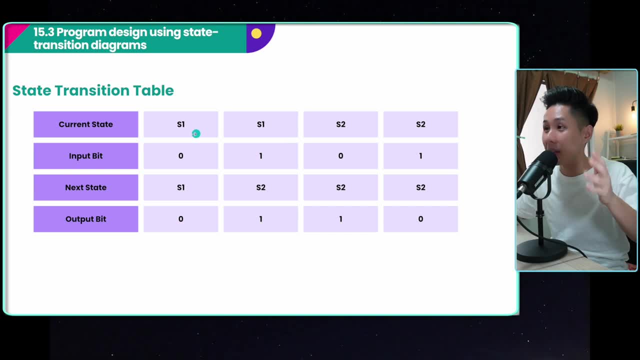 complement. so this is the method, of course, to explain what the question actually mean. but our goal is that we want to draw a state transition diagram. so to do that, we first need to do draw the state transition table. so s1 is the state where you output, whatever the user input, and state 2 is 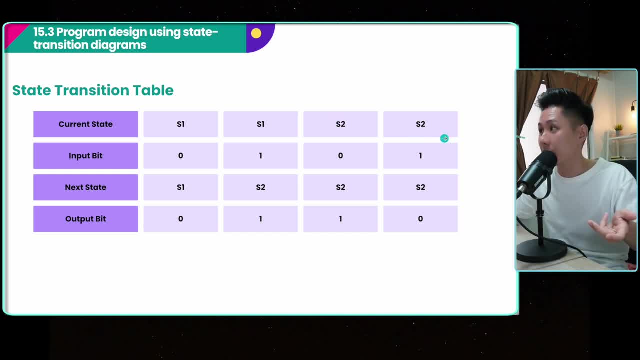 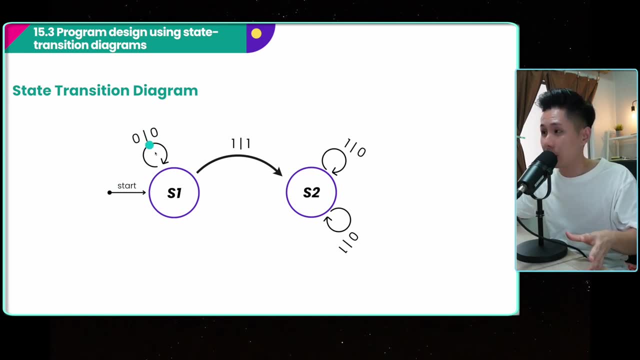 when you output inversely what the user input. so I want to show you in this diagram it would be a lot clearer. so at the beginning of the program, if the user entered 0, it's gonna go go back to yourself because this state says that your output 0. 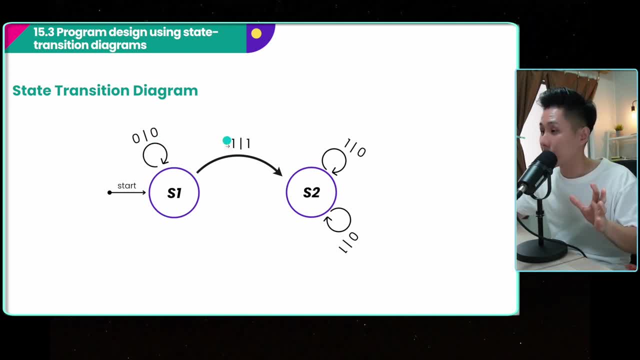 when the user output 0 until the user entered the first 1. this is when the program goes to from state 1 to state number 2. so if you enter 1, I'll put 1 first and in state 2, whatever the user input. 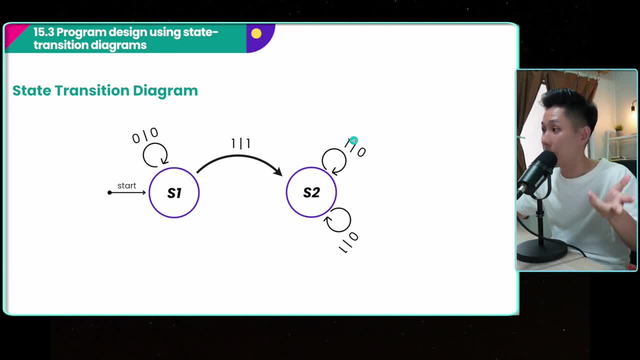 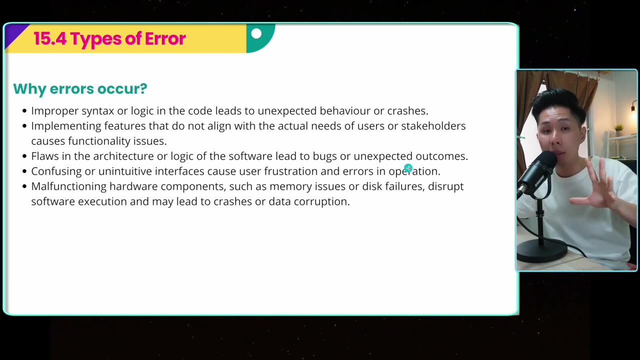 then you output whatever the inverse of the binary number until the end of the program. and hopefully, these three examples to give you an idea on how to draw state transition table and also state transition diagram. now, um, another aspect of software development is that errors could occur, and in this sub chapter we're 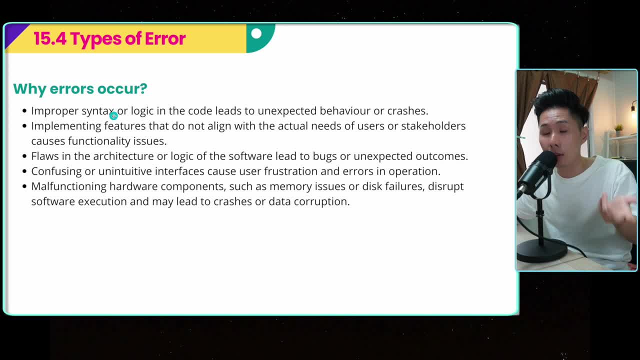 going to look into why error occurs and what are the different types of error that could appear. so i have a few reasons why error could occur: improper syntax, implementing feature that do not align with what the program requirement says. flaws in architecture. confusing or unintuitive interface, meaning the user don't know how to use it. malfunctioning hardware component. 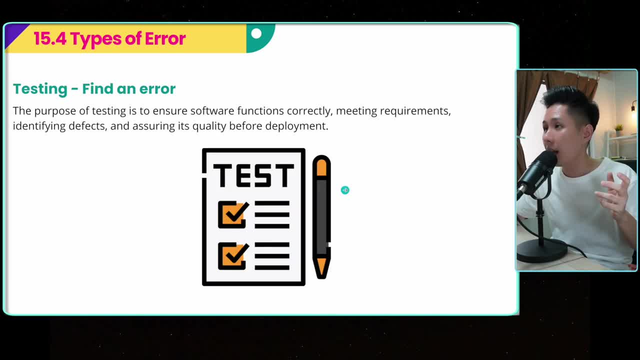 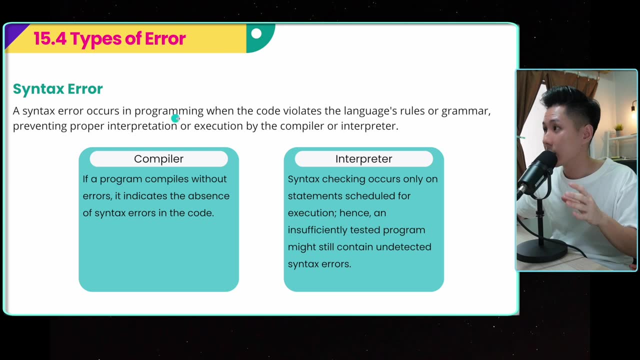 so these are the descriptions. feel free to read it yourself now. testing is a process that we use to find out all the errors in the program. all right, as implied by its name. there are a few errors that i want to go through. first one is syntax arrow. so it occurs. 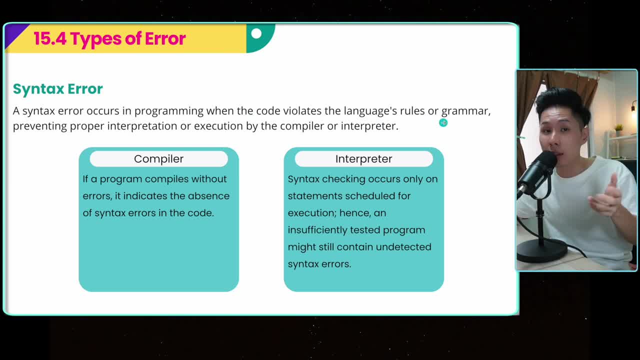 in programming when the code violates the language rules or grammar. so for example, in english, we can't just use: we is a good man, so that would be very wrong. right, this is um programming language also have the same rules. so if the programming programmers made this arrow, then it will prevent proper. 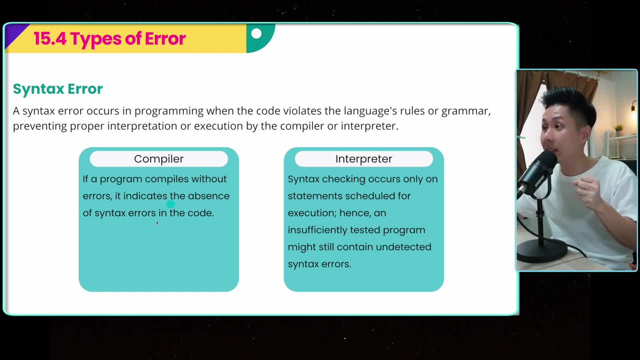 interpretation or execution by the compiler interpreter. and this is how compiler interpreter handle syntax arrow differently. so if a program compiles without arrow indicates the absence of synthetic error in the code, for, whereas for interpreter syntax checking occurs only on statement schedule for execution, hence on any insufficiently tested program might still contain. 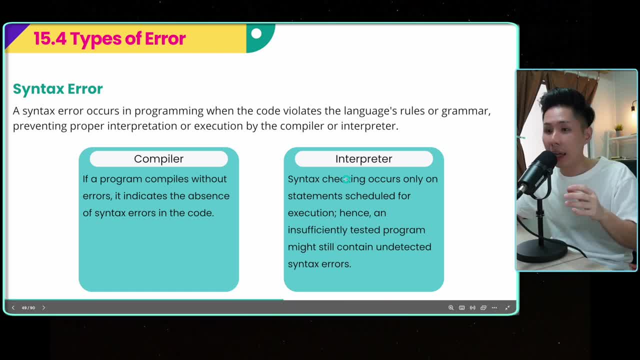 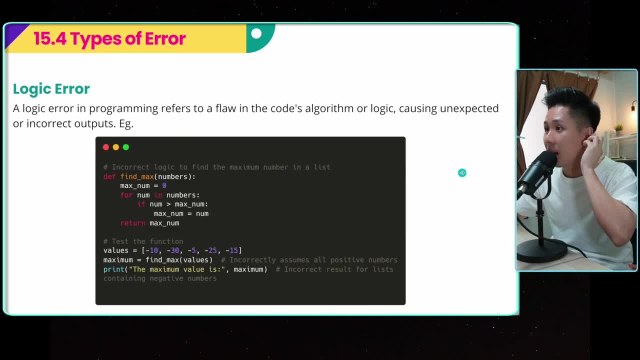 undetected syntax error. this problem occurs only on the communication schedule for execution, so the syntax error meaning it only run the code that is in that particular file, whereas compiler runs everything so that it can detect errors better. so another type of error is not so easily to detect. 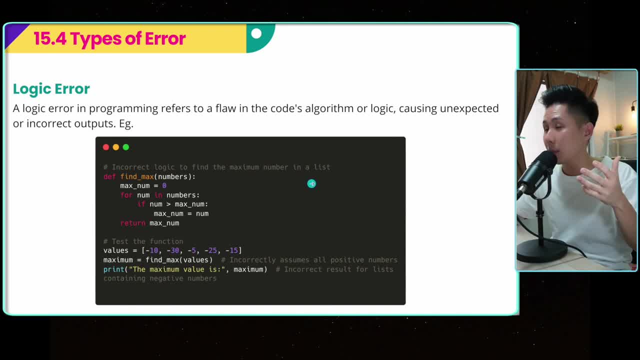 it's called logic arrow. you'll probably face a lot of this problem when you are coding. it refers to a flaw in the code algorithm or logic causing unexpected or incorrect output. so if you look at this code here- python code- it will look correct. until you run the code you found out that, hey, the program doesn't do what it's intended to do. 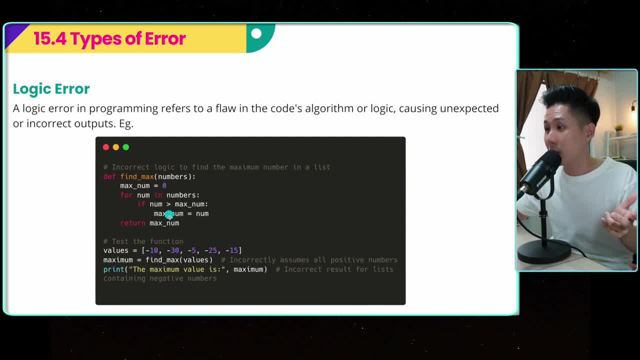 which is it doesn't find out the maximum, because if you run this code, it will still print zero. of course, if you know python, you will have know that the reason is because max number here is being set to zero. so this is why, when you put negative number to it, 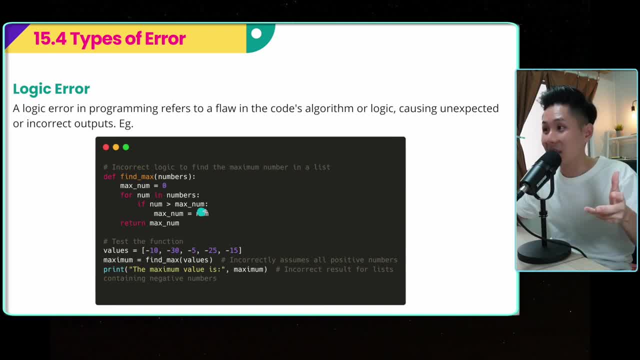 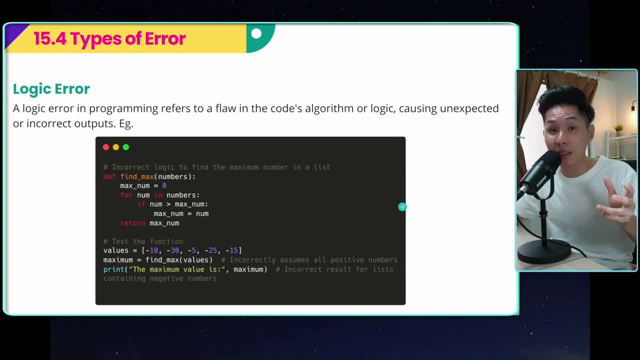 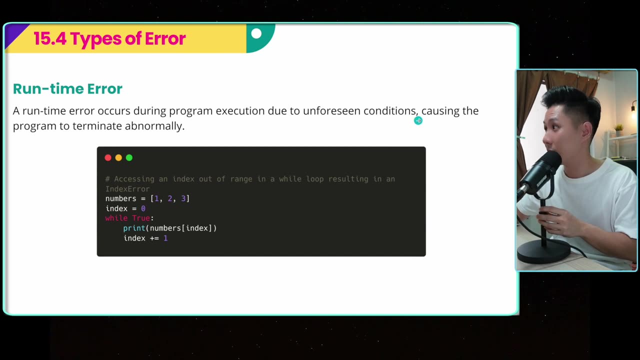 the algorithm will not detect that. oh, this is an arrow, all right, so this is called logic arrow, meaning the logic is wrong. therefore, the program cannot do what it's intended to do. another one is runtime arrow. it occurs during program execution due to unforeseen conditions, causing the program to terminate an abnormally, or it doesn't terminate at all, if you know python. 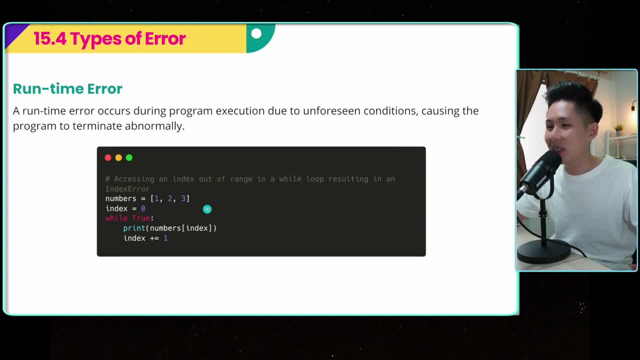 again, this is a code that i've written that will never stop forever, because i use a while true loop, meaning the condition will always be true. and don't try to put this code into your python, it will crash. so this is called runtime arrow, the error. that happens only when you run it. 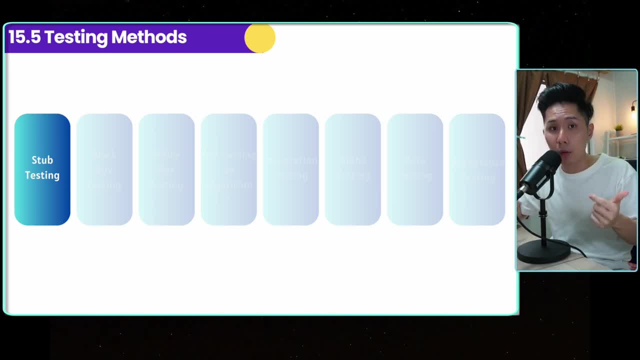 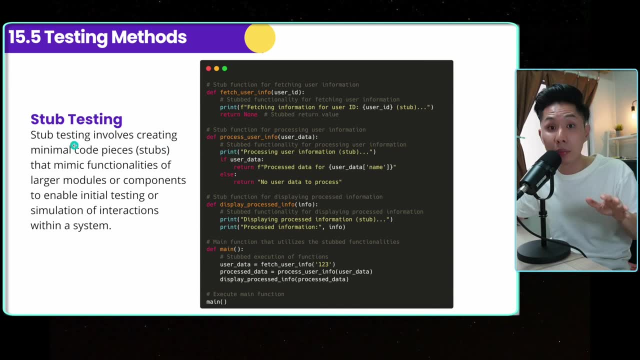 now we have talked about the different types of errors. now let's talk about what are the different types of methods. we can test out whether a program has arrow. first. one is called stop testing. it involves creating minimal code pieces that mimic functionalities of larger module components. so there are times when your program is very big, but then, um you, you're not at the 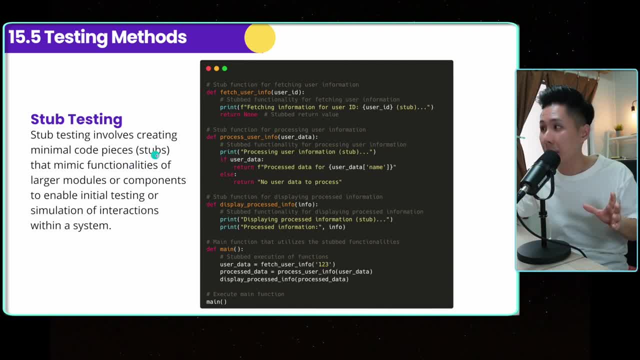 final stage yet, yet you want to test out whether it works properly with the model you created. so this is when you create something like called a stop code. if you look at all these functions here, they actually don't do anything. they just they are just printing. so this is just to complete. 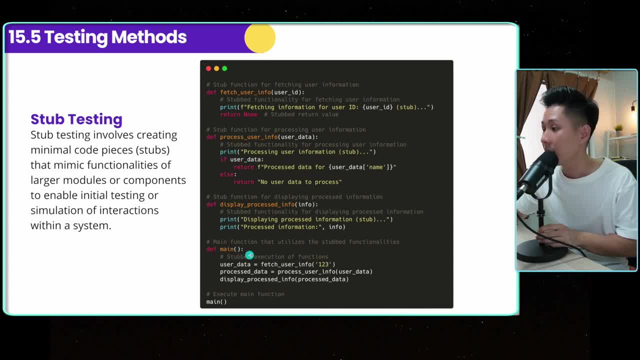 for the sake of completing the whole program. okay, and then what happened after everything works is that the programmer will go to each function and implement the functionality one by one, but then stop. testing is a good way for you to see the big picture of the program, how you want to structure it, and it will really make your coding life better. so the second type: 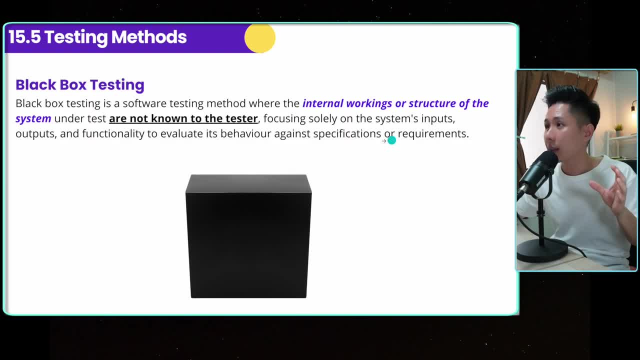 of testing is called black box texting testing, so it's it's a software testing method where the internal work is going to be done and then the software testing method is going to be done, and then the software testing method is going to be done, and then the software testing method is going to be done. 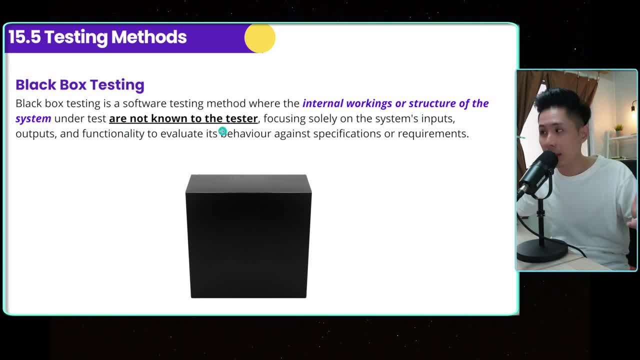 so the internal workings or structure of the system under test are not known like a black box here. meaning when the user tests the software they don't know what the code is like. meaning that when they test out the software they only focus on system inputs, outputs and 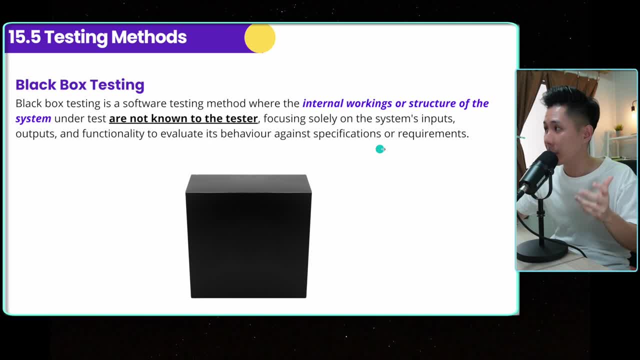 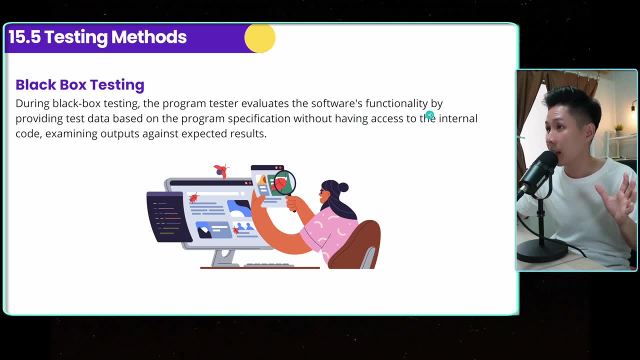 functionality to evaluate this behavior against specification or requirements. so during black block testing, this is what they will do. they will evaluate the software functionality by providing test data based on program specification, without having access to the internal code, meaning they can't change the code to solve their problem. all they do is that i give you this input and whether this 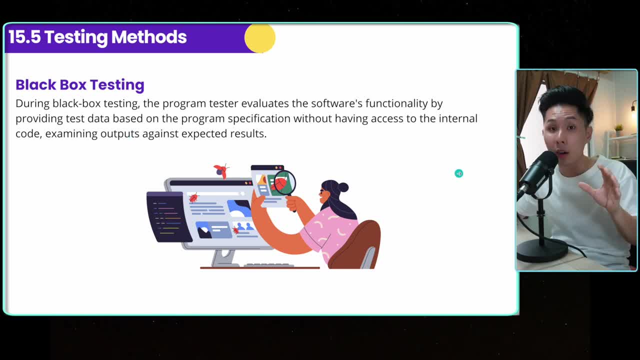 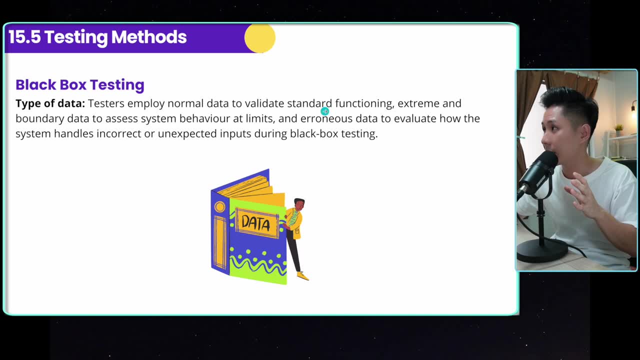 program can produce the output that is intended and that is called black box texting. so the type of data the tester will use: they will first use normal data to validate standard functioning and then they will use extreme and boundary data to assess system behaviors at limit to test limit. 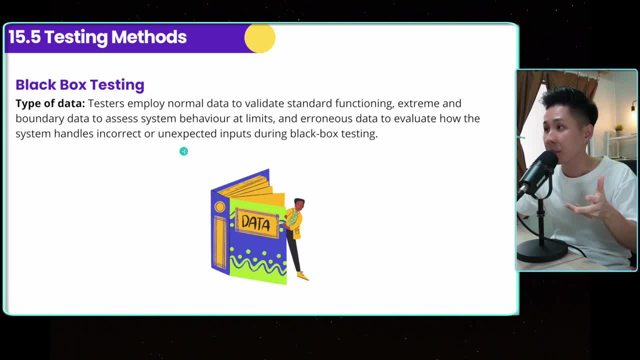 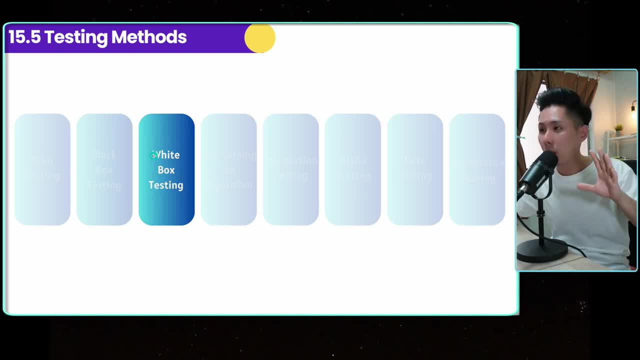 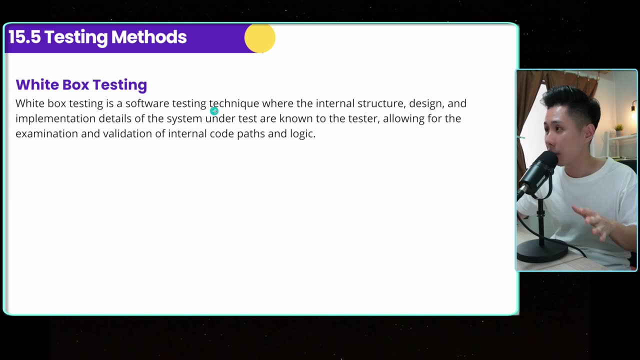 and erroneous data to evaluate how the system handles incorrect or unexpected inputs. so that's black box testing: the user doesn't know what's happening inside the software, whereas white box testing it is very clear to the user. it's a software text testing technique where the internal structural design and implementation details of the system under test are known. 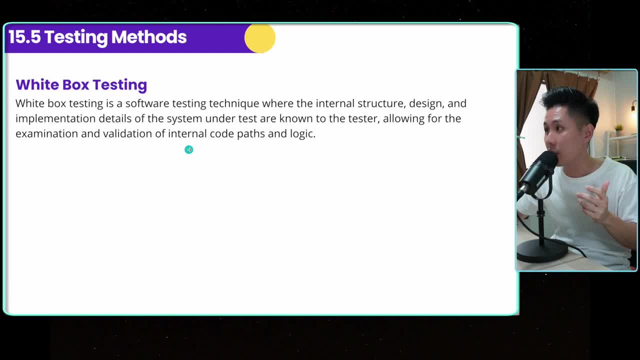 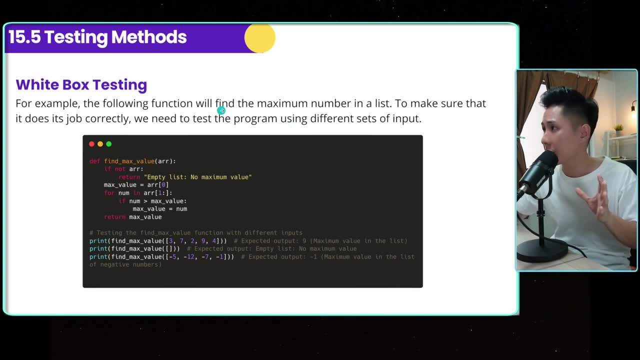 to the tester allowing the examination of validation of internal code part and logic is this is usually done by the software developers. so, for example, the following function will find the maximum number in the list. to make sure that it does its job correctly, we need to test the program. 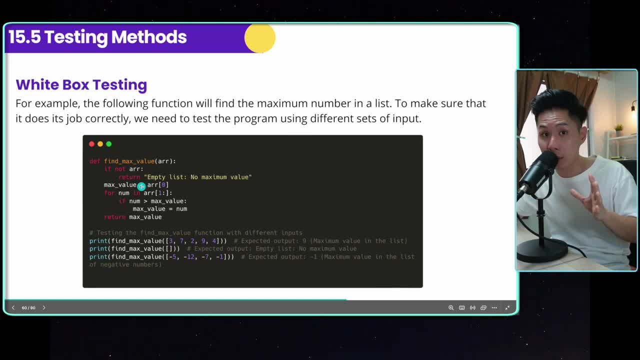 using different sets of inputs. so this function find the maximum value and to test whether it works correctly, you just try it out with different types of input, like a list that has all the positive number, a list that has all the negative number and a list that has no number. and you want 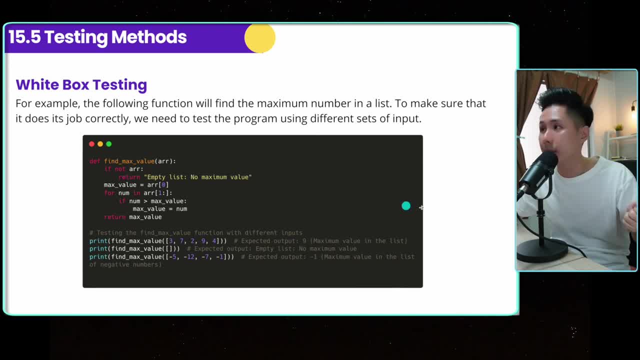 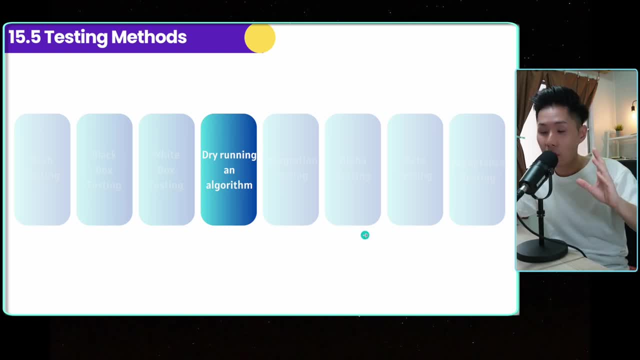 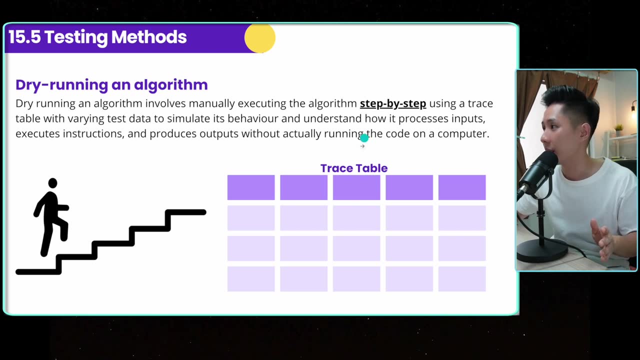 to see how your code will react when given different inputs. now the next one is interesting: dry running an algorithm, meaning, once you have written the code, you pretend that you are the computer and run the algorithm step by step, which is what i just talked about, and one tool that you need is called the trace table. 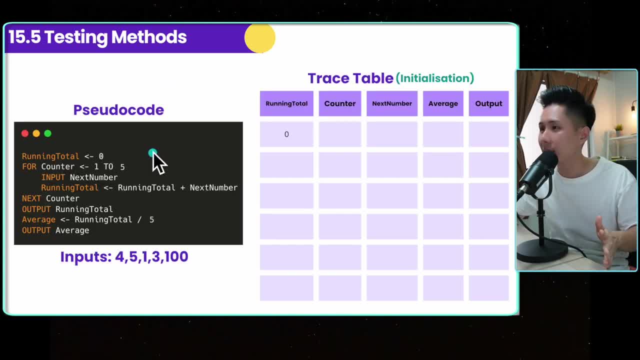 to drive, run your algorithm. let me show you. let's say this is our pseudo code and what it does is that it takes input from the user and calculate the average of it in a trace table. how it looks like is that it will have one column, or assign one column to each variable that you create. so if you look at, 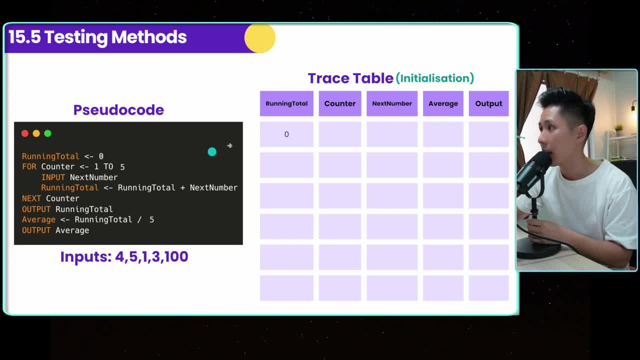 here the first line of code running total is the first variable. i assign a zero to it. so what happened is that trace table will trace the value of that particular variable at a particular step. so let's go through the code line by line. first line for counter one to five. so initially counter is initialized as one. 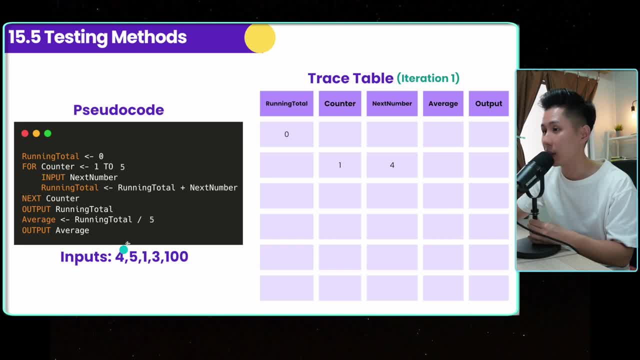 and next number. by the way, this is our inputs, the first one that we're going to input into the program: one, four. and the next line of code: running total equal to running total plus next number. all right, so you can see that zero plus four, which is equal to four. so i'm 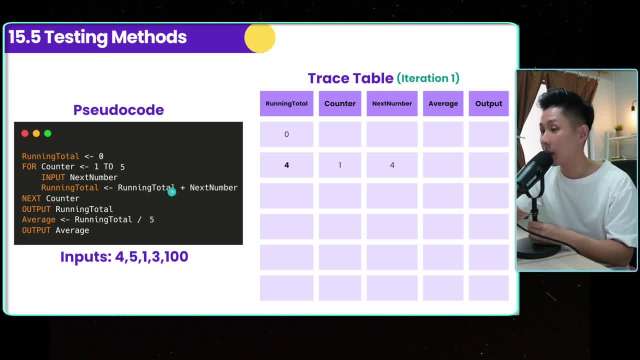 actually updating the running total variable here. so, because it's a loop that will continue to run it, it's going to be running for the next number to which is five, and the counter has been incremented to two, and then the running total will be nine, because four plus five equal to nine. so we 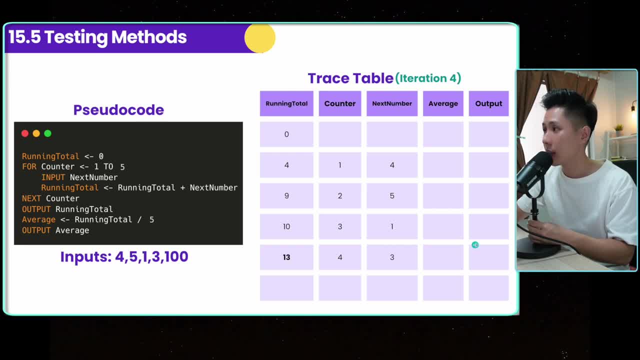 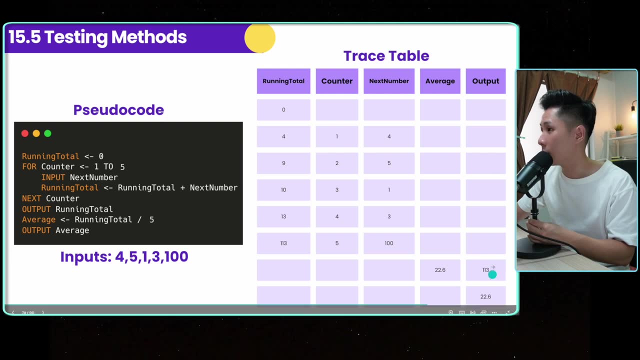 keep running the code and then track down what the count variable value is until we reaches the end of the for loop. you can see that running total is now 113 and then we'll output following this guy, and i will output whatever that is inside the running total and the average will. 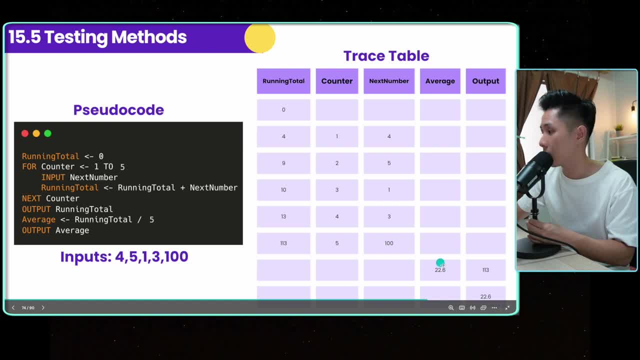 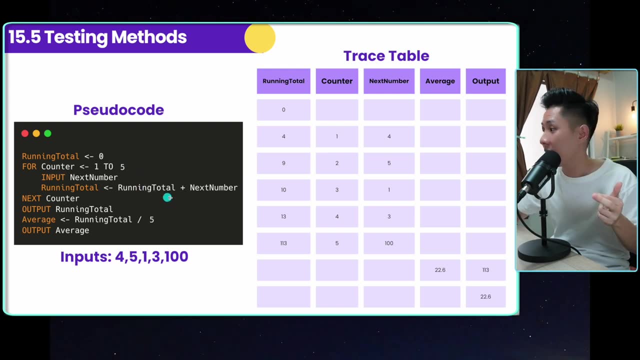 also be calculated by having running total divided by 5, 22.6 at the end of the program output average. so this is what trace table do. it mimics the program and then just run the program one by one to see one line at a time, to see what, how the variable value changed throughout the program. 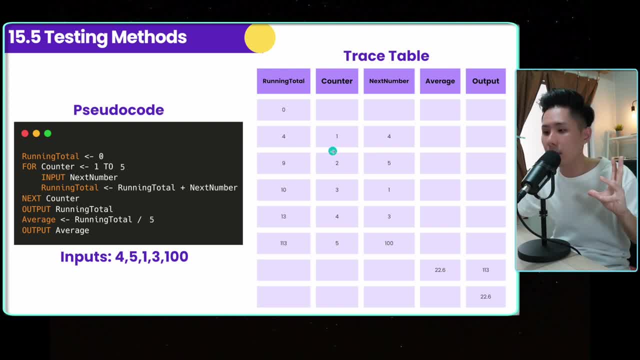 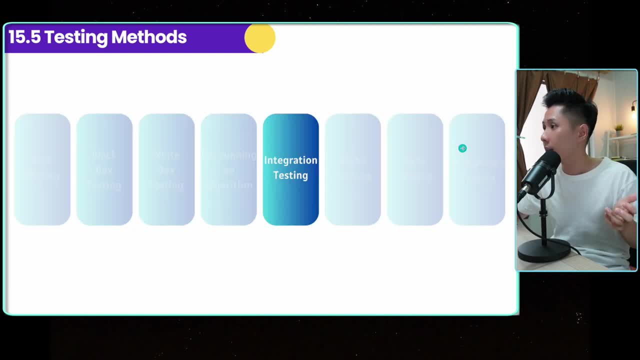 it will be useful when you are debugging. Let's say your program doesn't do what it intends to do By drawing a trace table. you know what went wrong. okay, So that's trace table, dry running an algorithm. The next way we can test a program- integration testing. 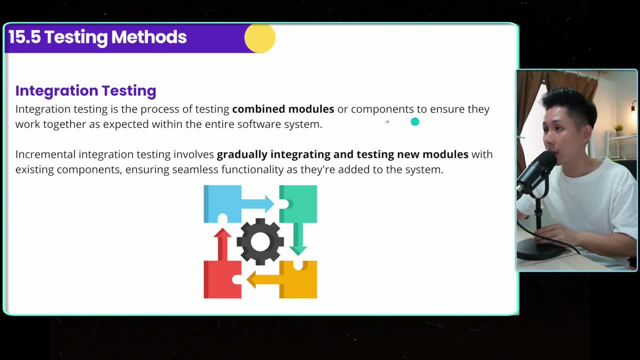 It is the process of testing combined modules or components to ensure they work together as expected. So in Python, we learn how to write function one by one. Think of integration testing as that. when you what happened when you combine all the functions that you have written? does it still work properly? 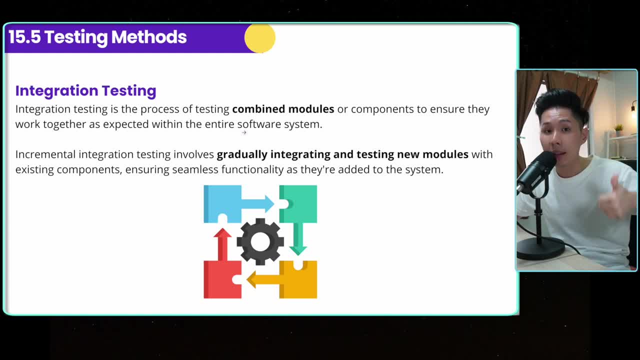 And for bigger software it could be that when they combine the front end and backend development, the code for that. So incremental integration testing involve gradually integrating and testing new module. So this is another method. incremental integration testing meaning we add one module at a time to the whole program. 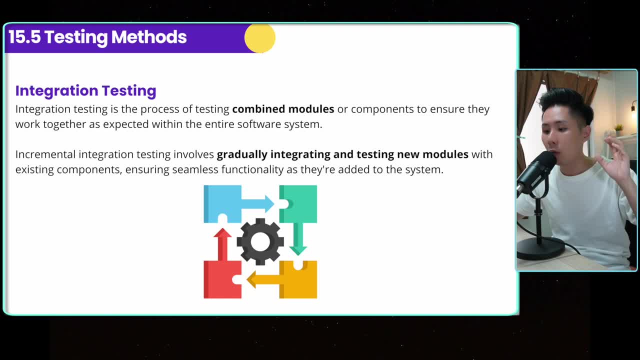 and then run it. add another module, run it And we see what is the. if, let's say, an error occurred, we can identify which module is causing the error And then we can focus on fixing the error in that particular module instead of going. 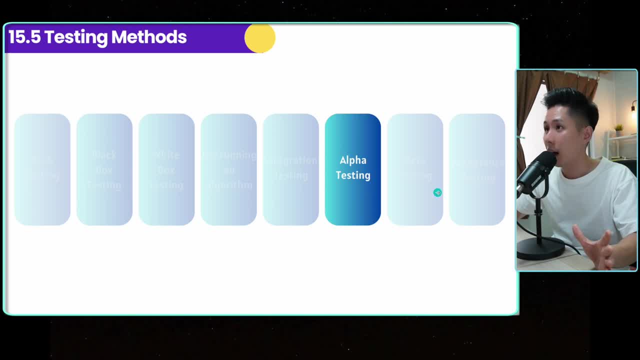 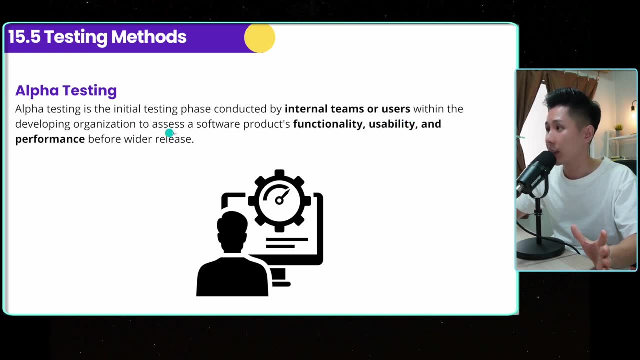 through the entire code base. Next one, alpha testing. It is the initial testing phase conducted by internal teams or users within the developing organization to assess the software- Meaning the team that developed the software- before they launch it to the public. they do an alpha testing, meaning they test it out. 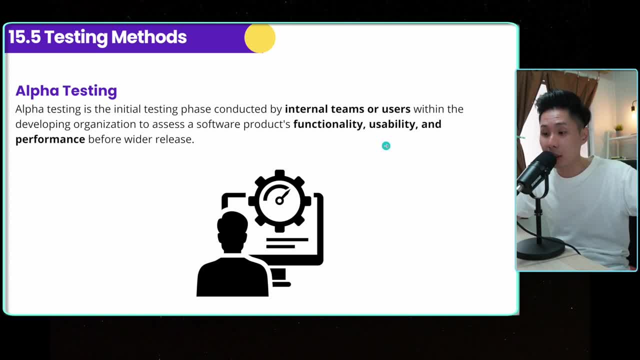 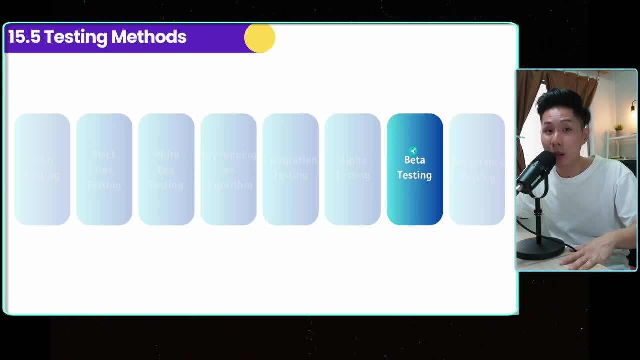 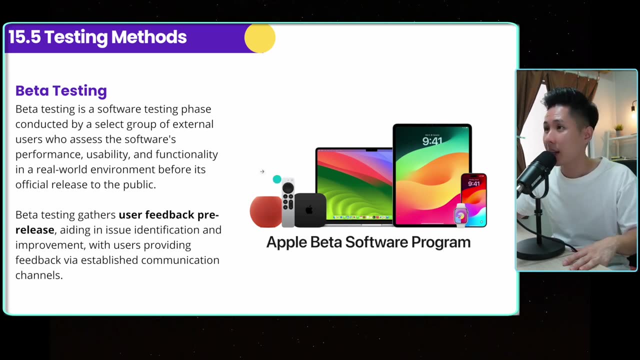 themselves. and of course, this is still not very effective. because you know your code, you might not do something that will crash your program, And this is why developers also come up with another tool called beta testing. Most of you might be familiar with the Apple beta software program. 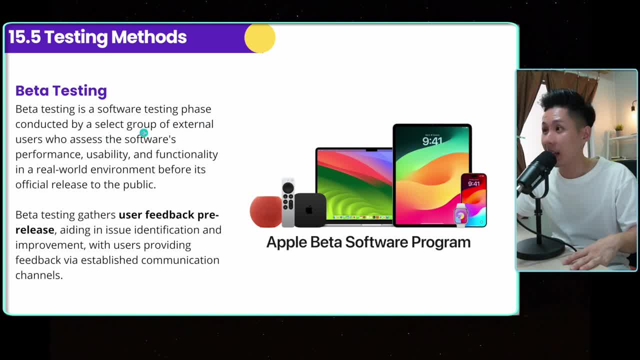 So this is a software testing phase conducted by a select group of external user who assess the system performance. So what happened is that once you publish a software you like, I said, you can test it out. you can test it out, launch it to not everyone. 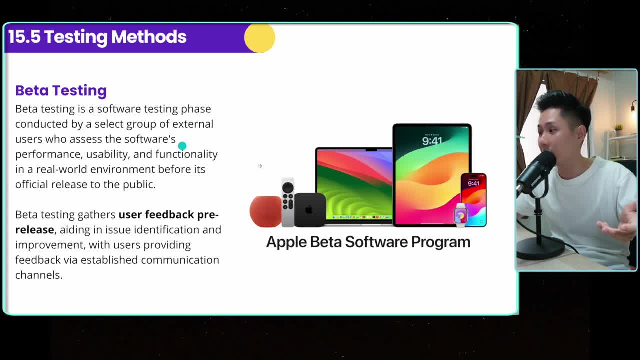 but then a selected group of users who have signed up for this For Apple program. I believe you need to sign up to just be the first one that tests out the new iOS system, But then the reason why Apple wants to do this is so that user can give it feedback on what went wrong. 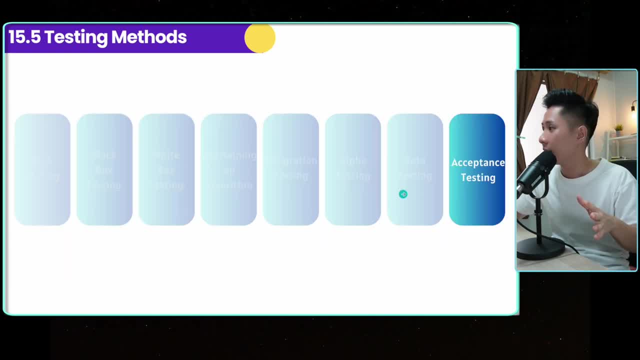 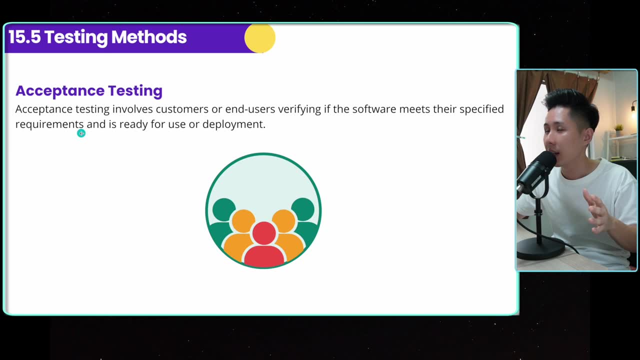 Okay, this is what stating here. beta testing. Last one, acceptance testing. It involves customers or end users verifying if the software meet their specified requirements And it's ready for use or deployment. meaning, acceptance testing wants to test whether the software is accepted. 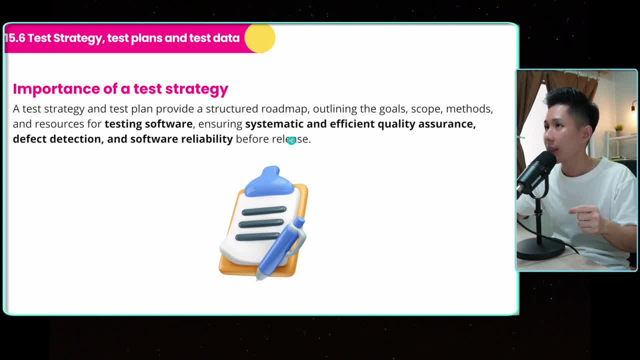 based on the user requirement here. Now let's talk about test strategy. So there are many different test methods, testing methods, So which one should you use? That's when a test strategy comes in. It provides a structured roadmap outlining the goals, scope, methods. 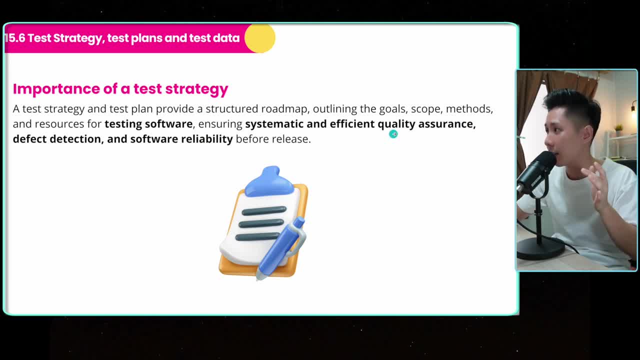 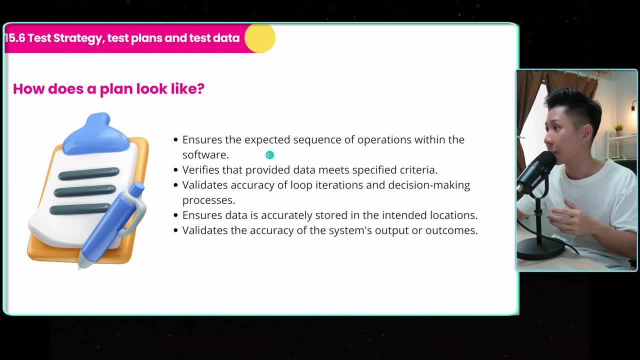 and resources for testing software, ensuring sustainability, systematic and efficient quality assurance, defect detection and software reliability. So how does the test plan look like? It ensures the expected sequence of operations within the software. verifies that the provided data meets specified criteria. validates accuracy. 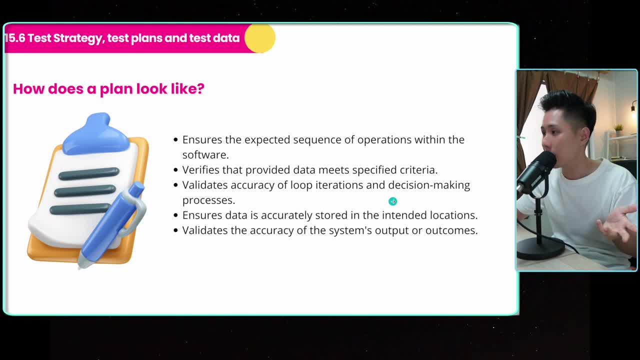 of loop iterations, meaning that it ensures that there's no runtime error. It also ensures data is accurately stored in the intended location, validates the accuracy of the system outputs or outcomes. So there are a few ways to carry out this test. First way is using data. 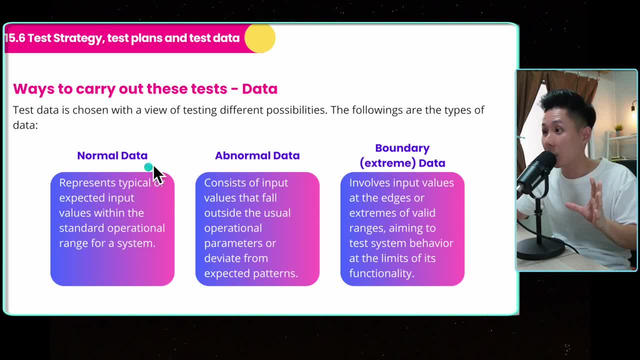 So there are different types of data that we have gone through just now. First one is normal data, Like what is the normal, typical data that the program will receive. Abnormal, as implied by the name, like data that is not supposed to be input by the user. 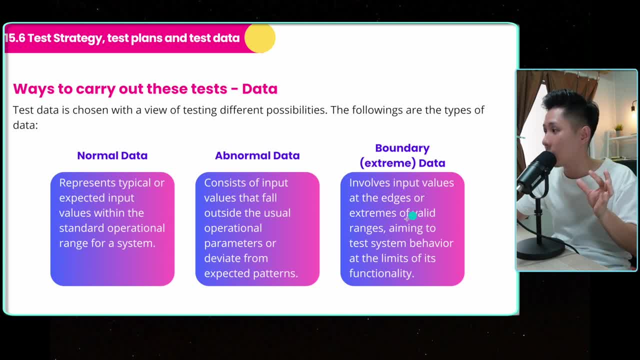 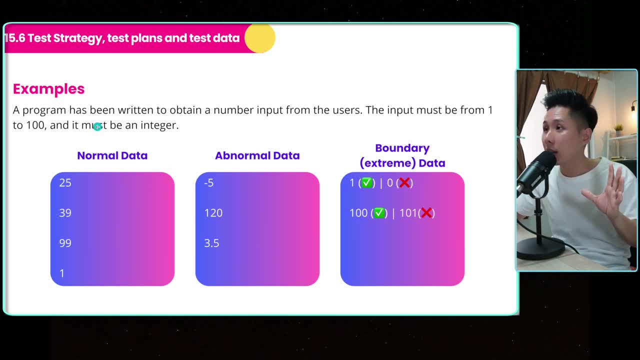 Boundary meaning input value at the edge, edges or extreme of valid ranges. It could be hard to understand using the definition, So this is why I created an example here. So let's say a program is written to get a number input from the user. 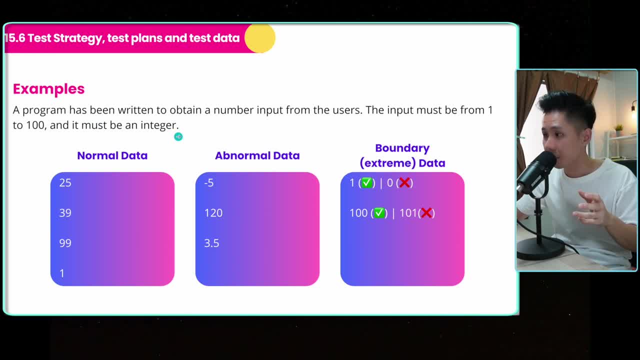 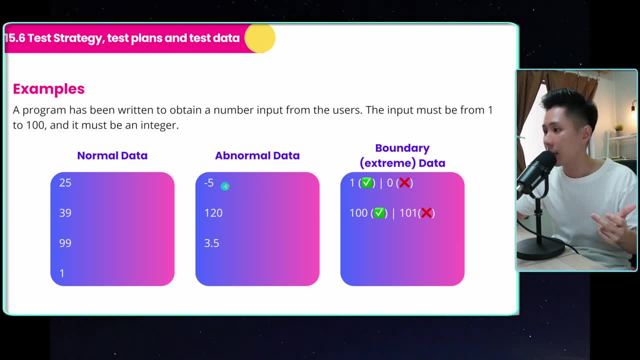 And the input must be one to a hundred and it must be an integer, So normal data will look like this: All the numbers that are within range And normal data could look like this: Like this is a negative number. This is bigger than 100. 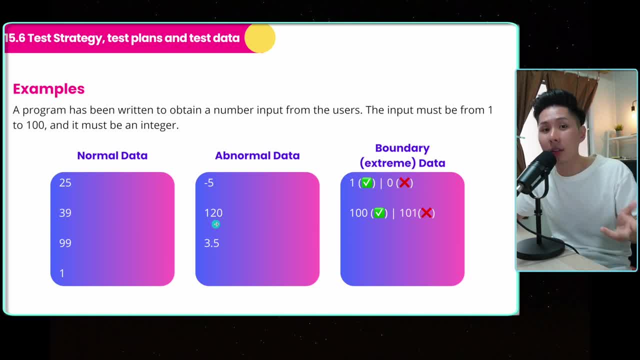 And this is not an integer To test out just how the system will react. And boundary data is basically the data at the boundary, using one zero. So these are the boundary data, because they are just at the edge of the accepted range, And 100, 101.. 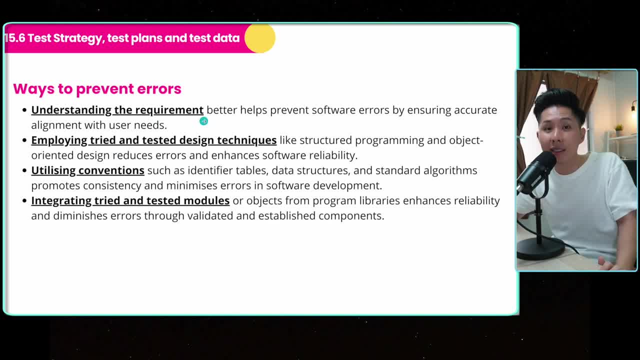 So ways to prevent error: understanding the requirements. This is important. I believe this is the most important. when you're developing a software, You don't want to create something that the user doesn't want to use, That the boss doesn't want you to do this. 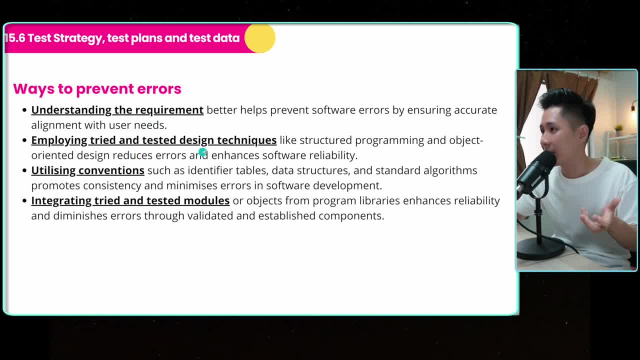 So you want to understand the requirement Employing tried and tested design technique, like structured programming and object oriented design, Which is something we'll talk about in the next few chapters- Utilizing conventions like the identifiers tables that we look in. We look at that- the pseudocode chapter. 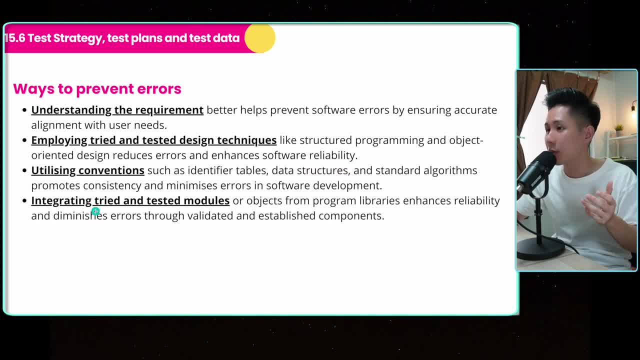 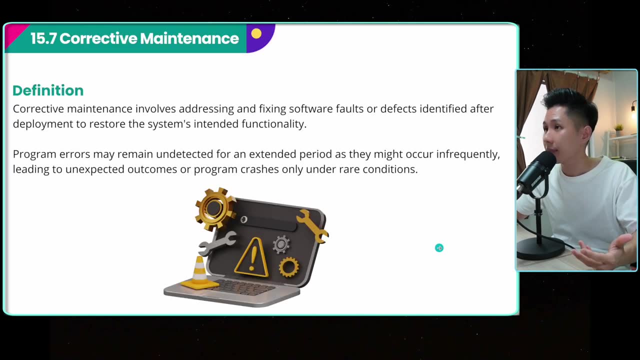 They use proper data structure And integrating tried and tested modules, Meaning we only integrate modules or functions that have been tested into our main program So that we can reduce the probability Of a program having an error. Now we're looking to the last part of the video. Which is the three different types of maintenance. Which is pretty easy: Corrective maintenance, So once the product, once the software has been shipped, There usually needs to be maintenance, usually needs to be done. And the first type is called corrective maintenance. 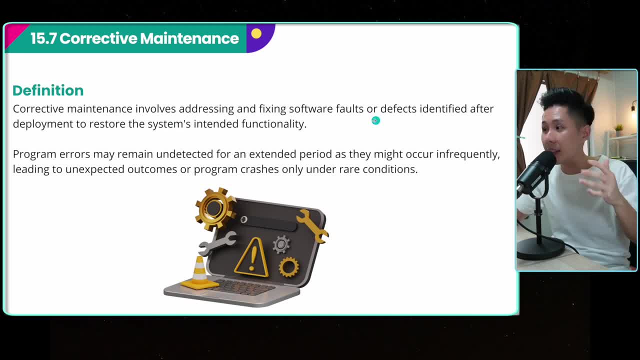 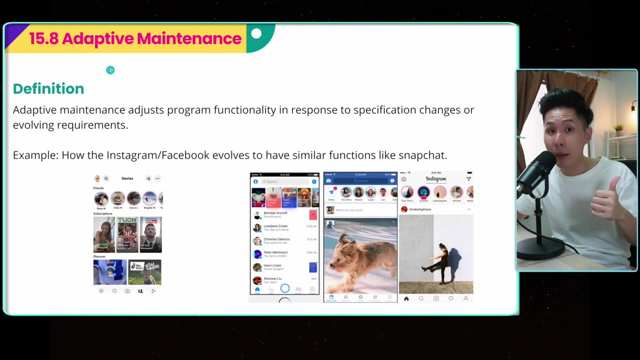 It involves addressing and fixing software fault. Basically, if your program has a bug, Then your role as a programmer Is to maintain it by solving this bug So that it doesn't happen that frequent. So another one is adaptive maintenance. It adjusts program functionality. 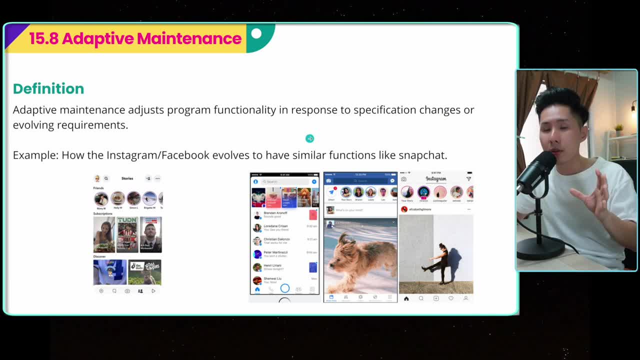 In response to specification changes. So remember when I told you about the program development life cycle. They just programmers will just keep going through the circle To add new requirement, new design, new code, new testing method. So one example for adaptive maintenance I see is how